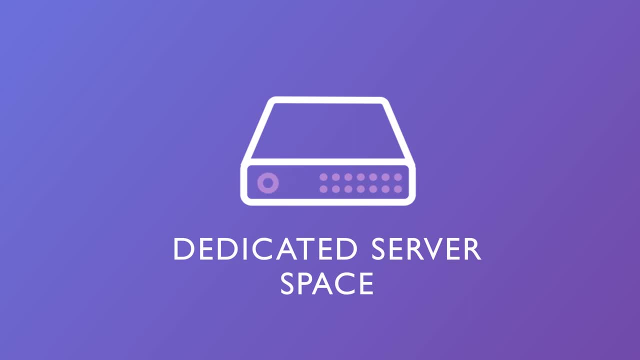 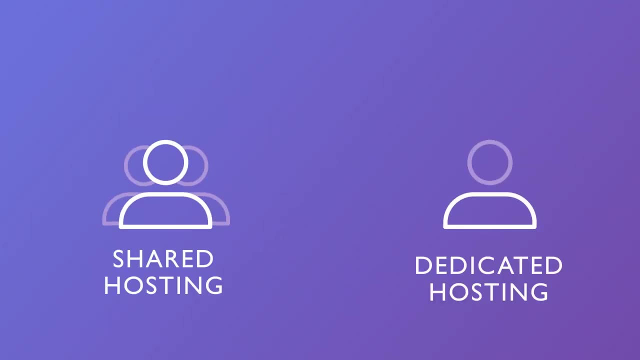 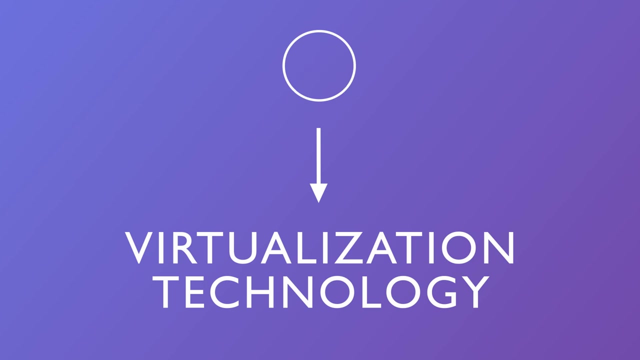 VPS hosting combines features of both shared and dedicated hosting, But the difference is that VPS uses virtualization technology to divide a single physical server into multiple independent virtual servers, giving your website the ability to operate and manage multiple virtual servers. So VPS hosting is a great way for you to get a dedicated server space just for you, with a 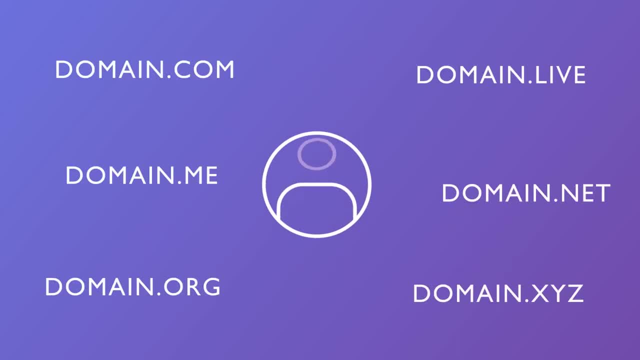 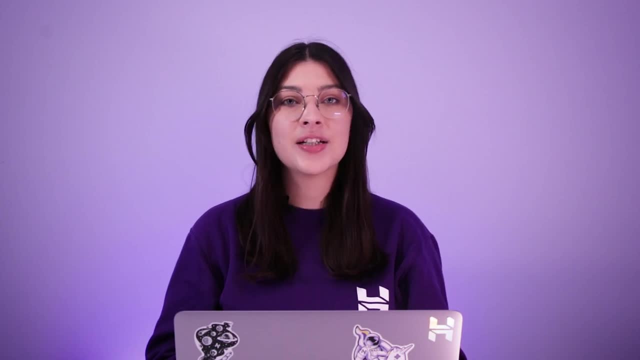 reserved amount of resources and memory. You can also create a dedicated server space for your site, So let's get started. Running a VPS lets you set up a website within secure space with guaranteed resources that you don't have to share with other users. Also, with VPS hosting, you have the same root-level access. 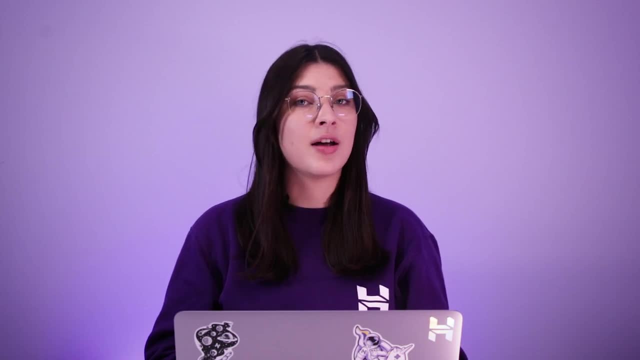 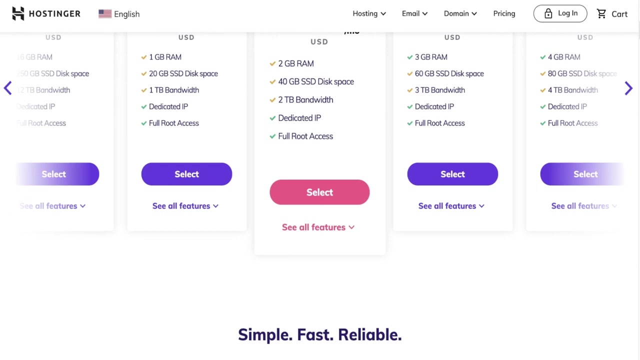 as if you had a dedicated server, but at much lower cost. That allows you to configure your site from the ground up, meaning you can install any software application, create a design and so on. However, one of the biggest difficulties of VPS hosting is managing your entire server environment by yourself, So you 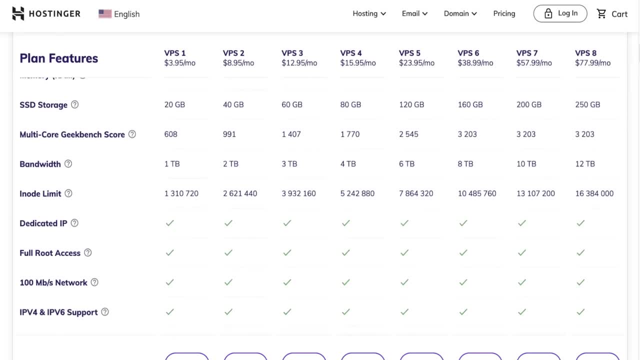 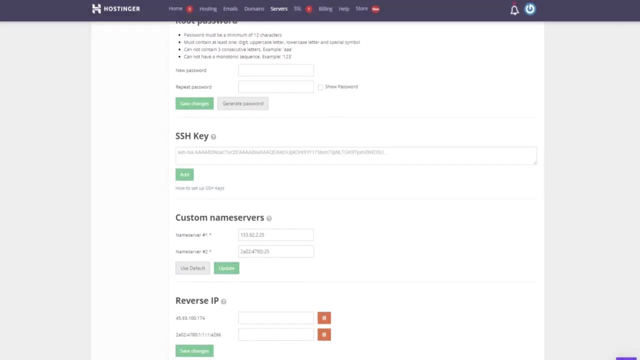 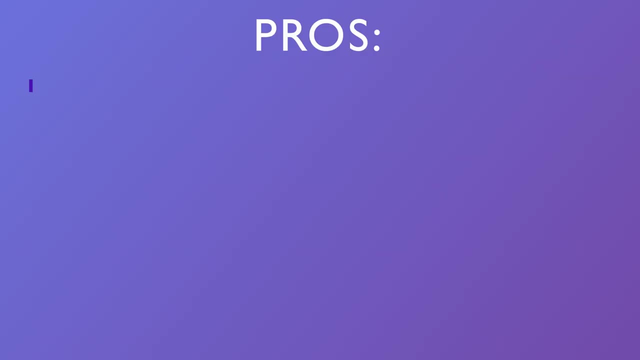 have to have experience in web development. If your virtual server is not configured and maintained well, you may face security or performance loss problems, But you can always hire a system administrator to help you out. Alright, let's break down VPS into pros and cons. 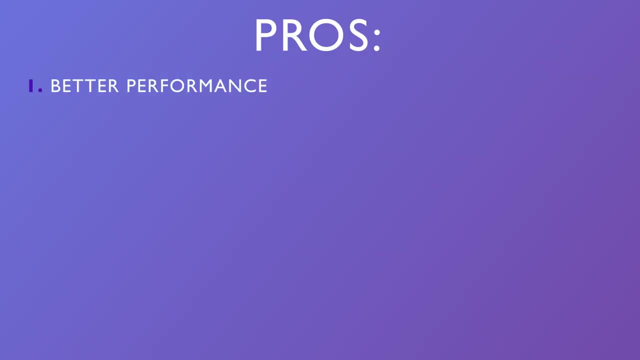 So the pros are: The performance is much better than a shared hosting server. Traffic surges on the other websites do not affect your performance. You get root access to your server. You have a better privacy and security, as your files and databases are logged from other server users. 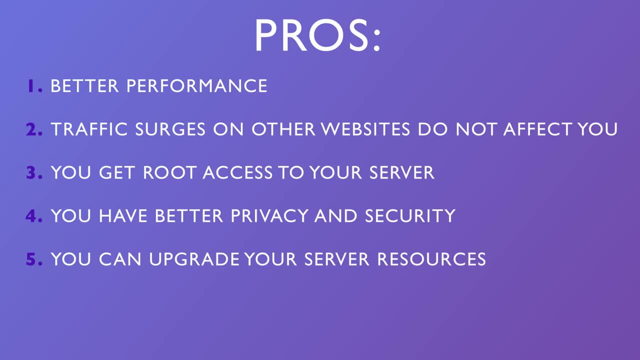 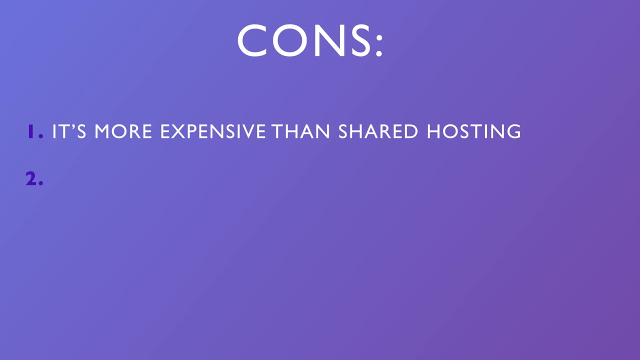 You can easily upgrade your server resources, such as RAM, CPU, disk space and others. It's less expensive than a full dedicated hosting plan And the cons are It's more expensive than shared hosting. Improperly configured servers may lead to security vulnerabilities. Technical and server management knowledge is a must. 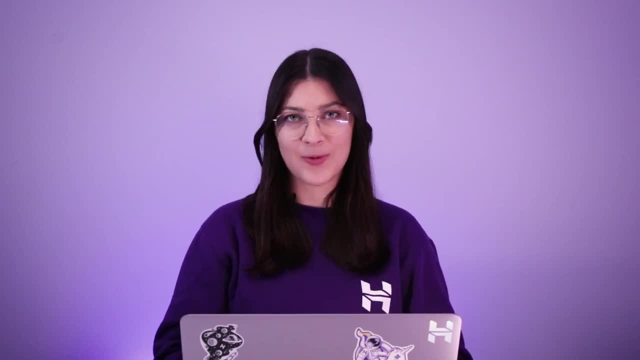 Alright, and that concludes today's video. It was easy, right? But if you have any questions, don't hesitate to leave your comment below and I will get back to you. And, of course, if you liked this video, give it a thumbs up. 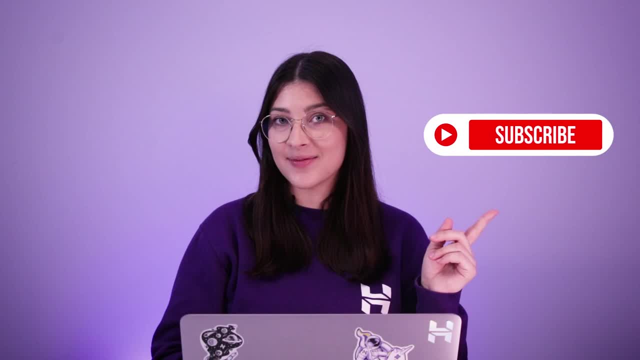 share it with friends and subscribe to our channel for more content Till the next time. Thanks for watching and have a great day.